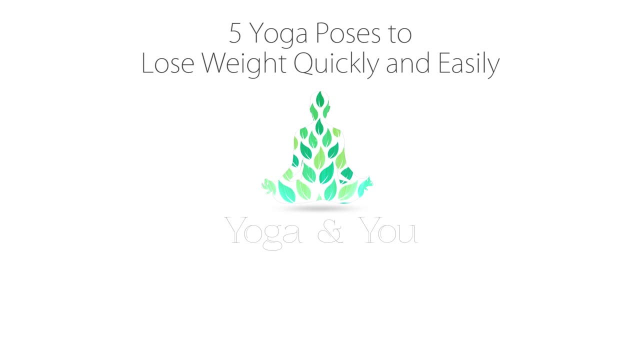 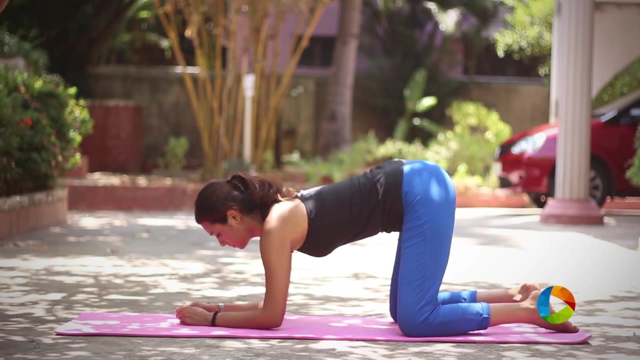 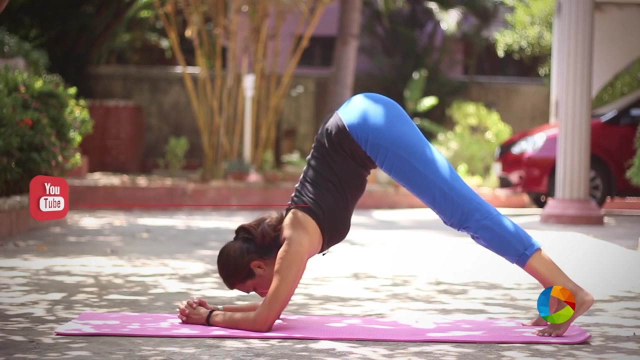 So now, once you are ready, just come onto your knees and placing your elbows really firm and nice, interlock your fingers and take few deep breaths, curl back your toes and, as you exhale, just slowly lift your knees and hips away from the mat and putting your 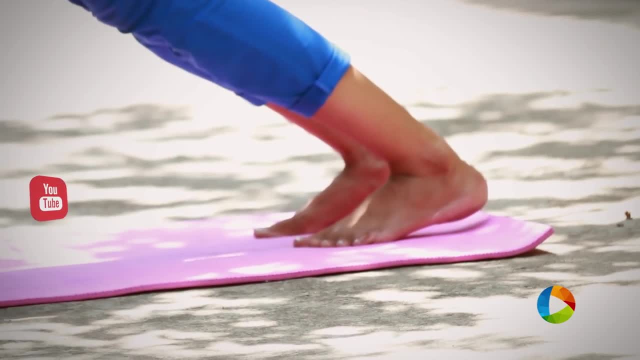 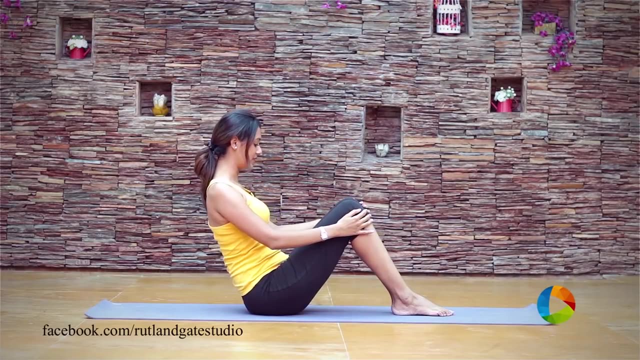 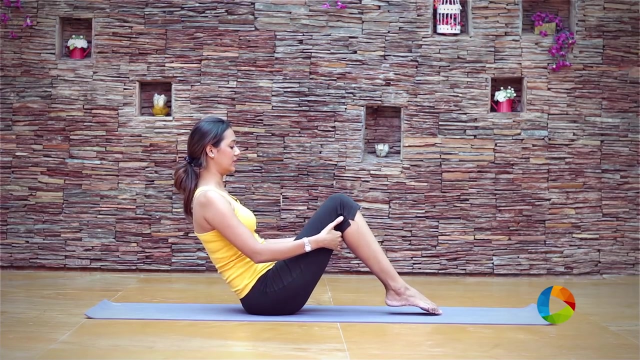 head down, breathe normally, inhale and exhale. make sure your breath is really normal. So roll your shoulders back and slowly lean all the way back, just like this, so keeping your back strong and nice and sturdy. And from here, as you inhale, lift your legs slowly. 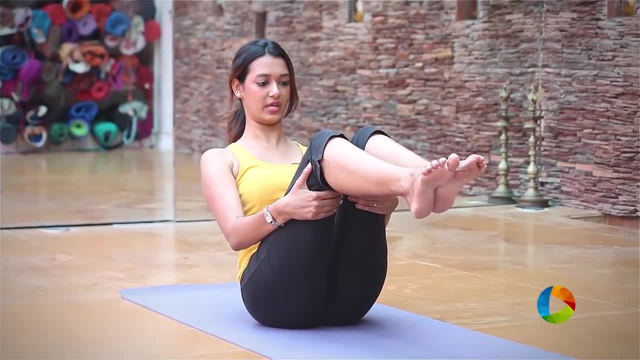 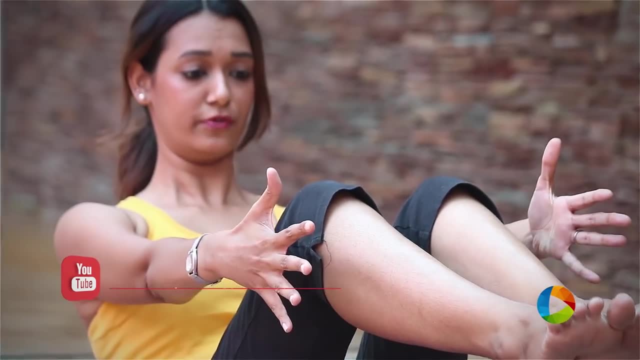 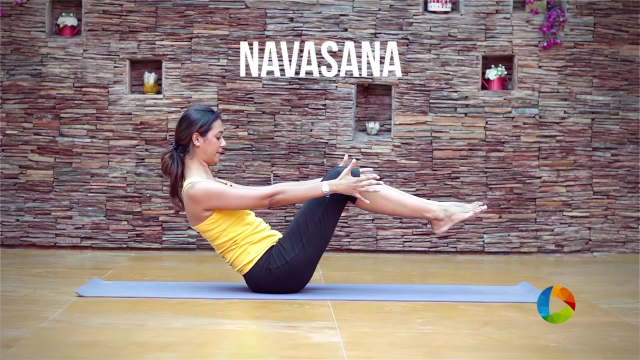 off the mat, Inhale, lift your legs all the way up, Slowly release your arms to the sides of your body and hold the posture, not your breath. Remember to breathe For five, four, three, two and one. You are going to place both your elbows right at the. 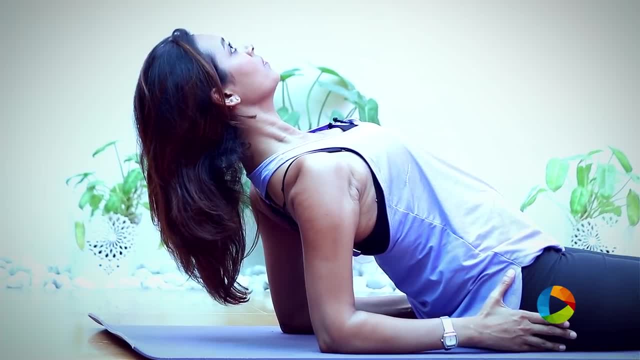 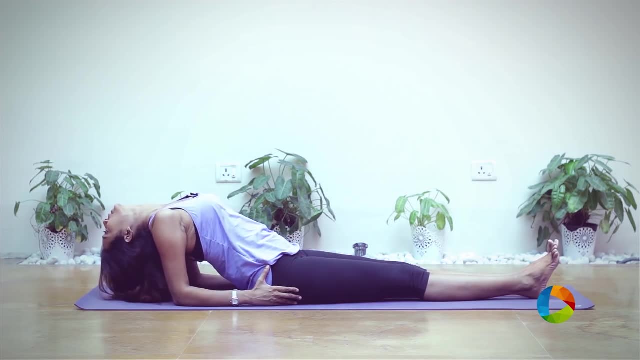 back. Open your heart first as you inhale and slowly as you exhale, drop the crown of the head all the way down to the mat. Now, from here. if you cannot reach the floor, you can always adjust by walking through your elbows. 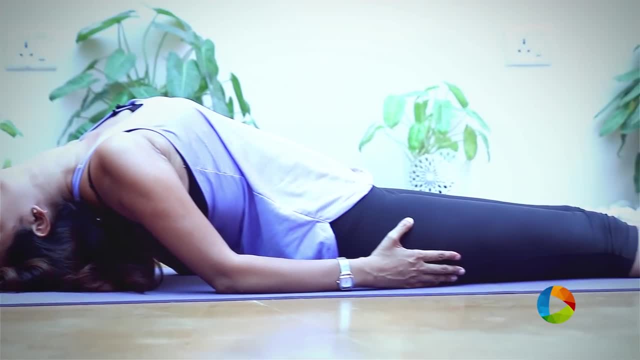 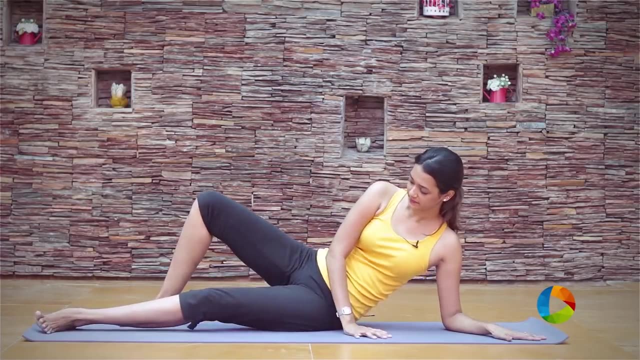 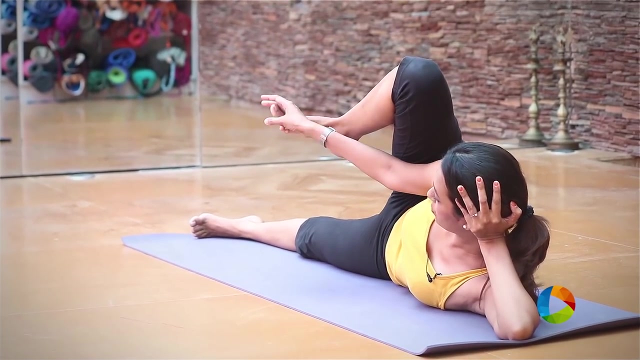 And stay here for a couple of deep breaths. Begin by lying down onto the side, Lying really comfortably down here. so support your neck, Inhale, lift your right leg up- Okay, and hold your right big toe with your right arm. 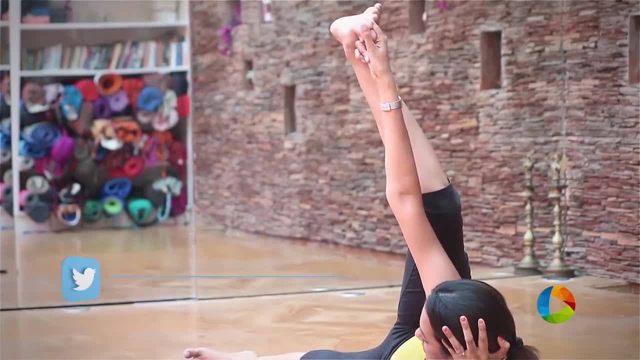 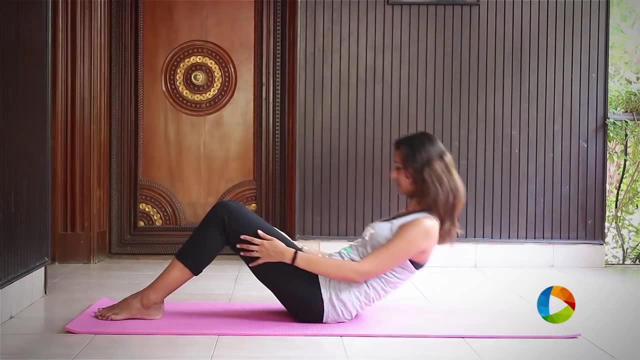 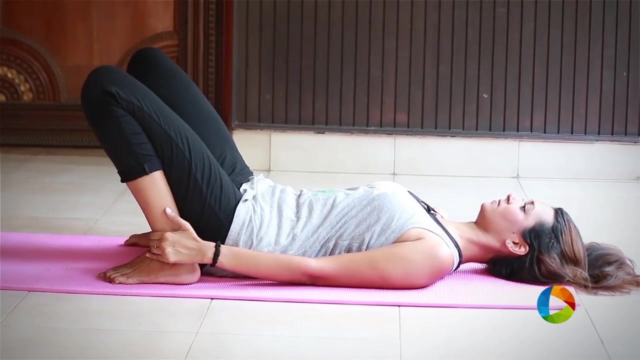 and slowly as you exhale, lift and extend your arm and your leg as well. Hold here, Begin to lie down on your back and place your heels as close as possible to your butt and hold your ankles. Make sure your thumb is outside and, when you are ready, slowly inhale and lift. 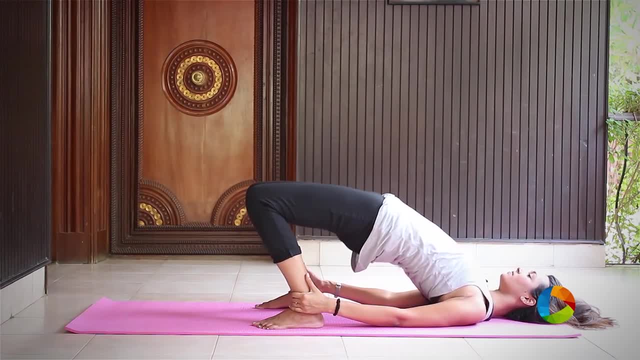 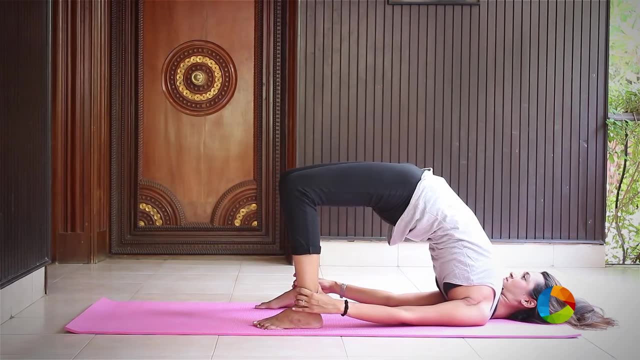 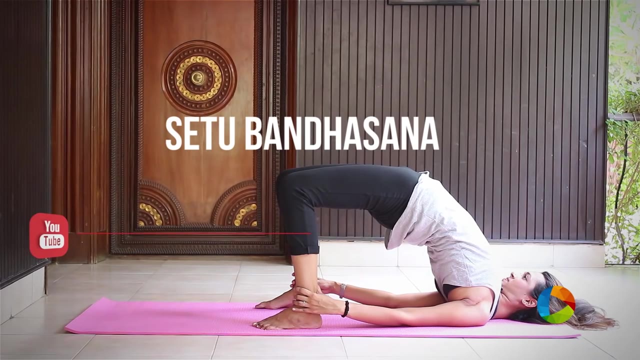 your hips all the way up. So try and reach as high as possible, but your breath should be in the normal range and stay here for a couple of deep breaths. Thank you so much for watching and I will see you in the next video.